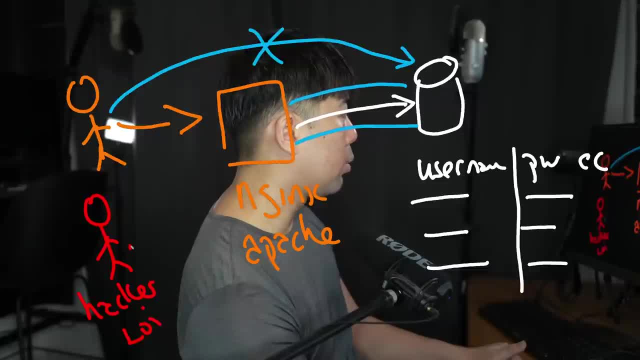 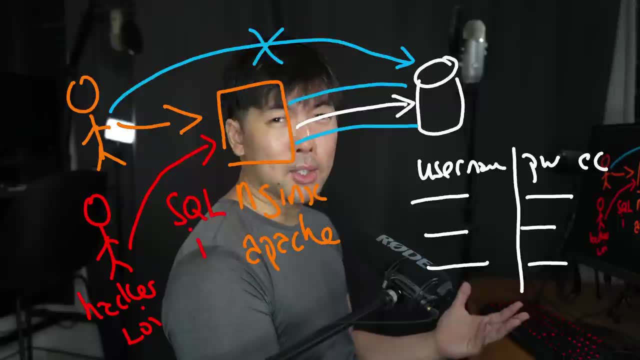 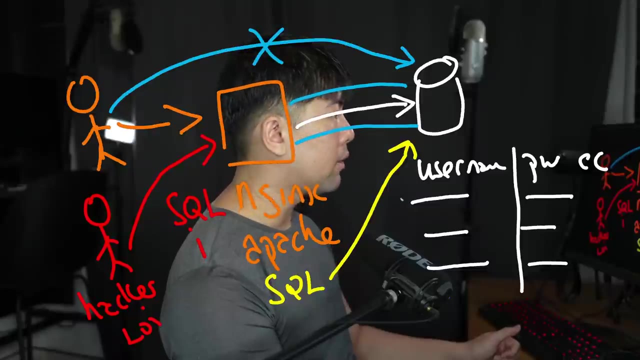 which is your best friend, your BFF, and here Mr Hacker Loy, would then have to target into the application server and has to inject what we call SQL injection. So now you'll be asking: what exactly is SQL? So what SQL does for us is that SQL sends instructions into the database to interact with it in order to retrieve 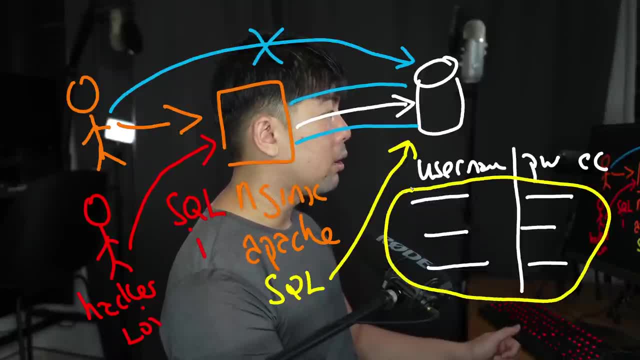 all these different usernames, Password fields and make them available into the application server, which can then run all these different logical checks. For example, did the user who entered a password does it match with the password over here under the username that's been supplied? 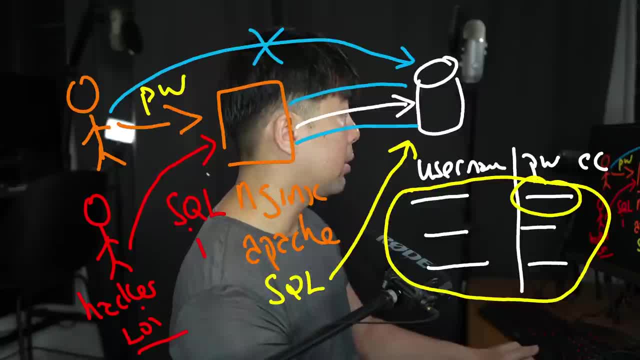 And going back to the hacker over here, what SQL injection is trying to do is to bypass some of these different logics so that we are then able to gain unauthorized access into the database listing down all these different usernames, passwords, credit card information from the backend system. 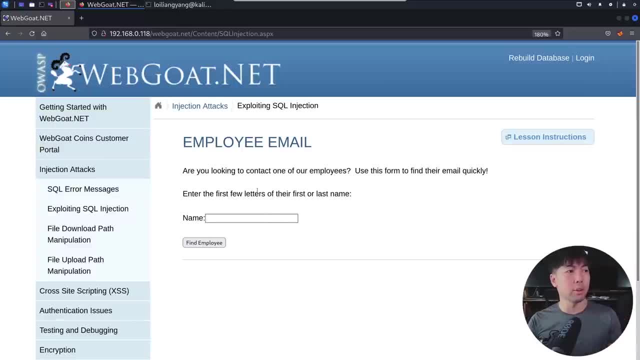 So right in front of us we have webgonet and here we have the employee mail and, of course, here it says the following: are you looking to contact one of our employees? use this phone to find an email quickly. So, again, as I've shared, there's a backend database to do the lookup for it. 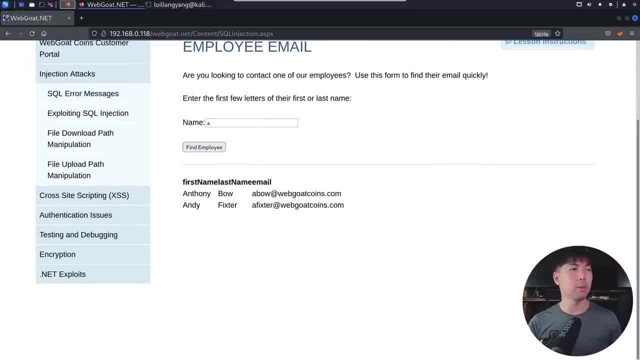 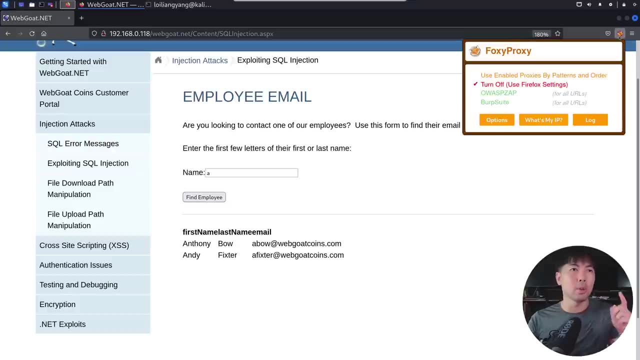 So we can enter a name, so I can start with A find employee and we can see right here we have first name, last name and email address. So what we can do now is that there is a request heading into the server and what we can do is to go to the top right corner. 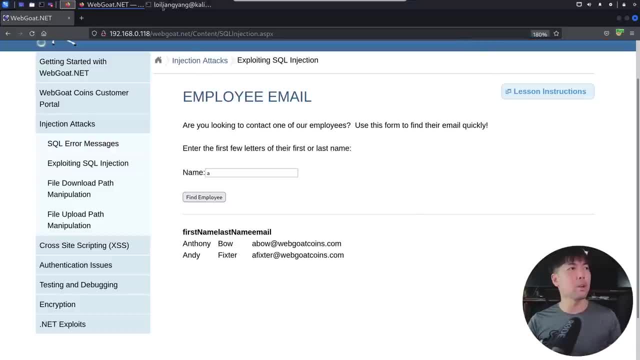 click on the Foxy proxy, click on the Burp Suite and once you're done with that, go ahead and open up a terminal and we can launch Burp Suite Right from here. so enter Burp Suite and here we're, starting a Burp Suite to be our interceptor. 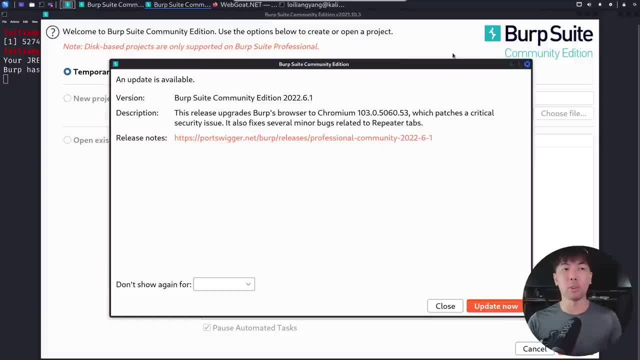 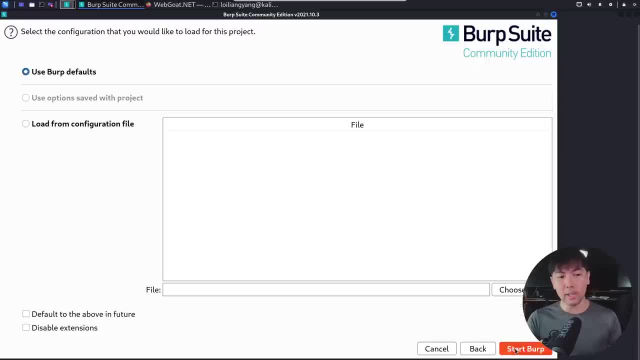 so that we can see all the different type of requests that are going over into the server and we can decide how we want to change up the request or perhaps even load the request to a separate software. So in this case, click next, start Burp. and now we are getting Burp Suite Community Edition started. 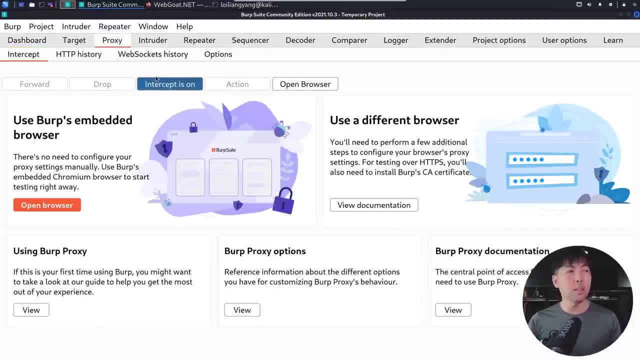 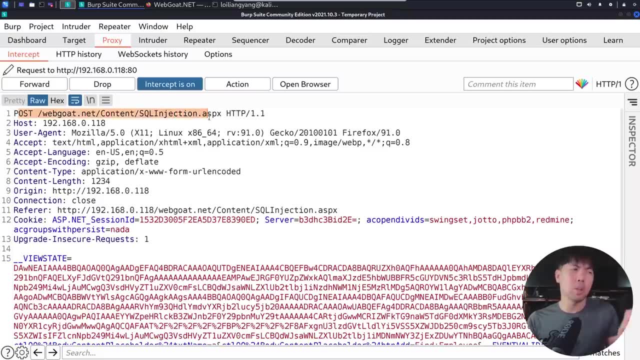 And go under the proxy tab and we can see the intercept is on. So once you have that, what we can do now is to go ahead and click find employee again and we can see the interception right here. So we have a post method going to SQL. 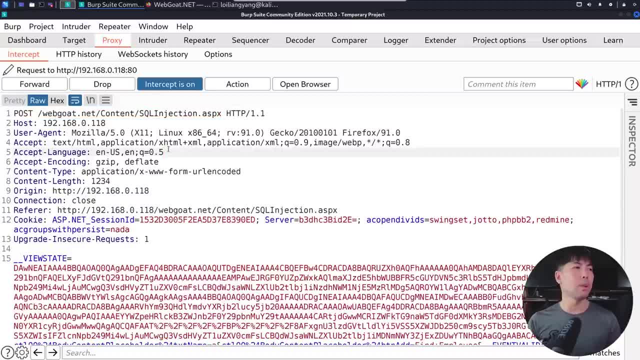 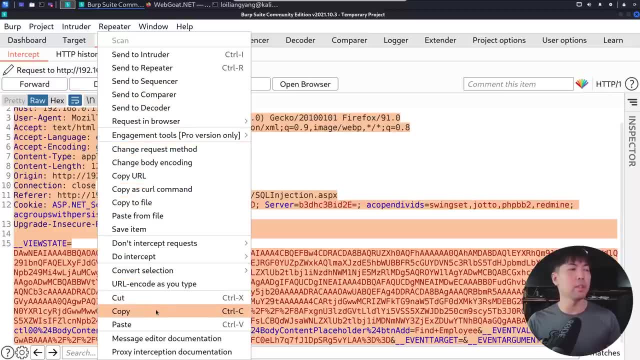 Injectionaspx. so what we can do now is we can literally copy everything right here. okay, You can do a right click and you can do the copy, or you can copy to a file, whichever the case is. so I can do a copy right here. 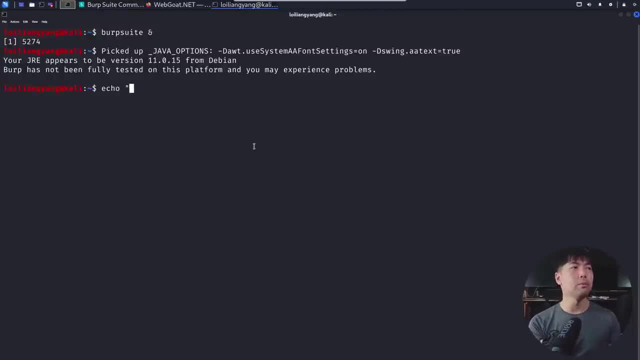 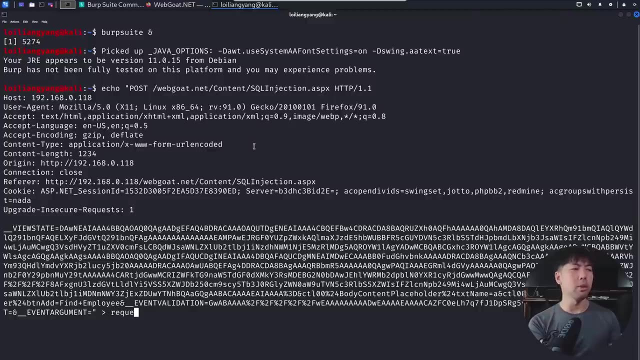 I can go back over into terminal and what I can do now is I can echo and I can copy and paste it over here and I can send this out to a file So I can enter, say, into a requesttxt: hit enter on that and I can do a cat requesttxt. 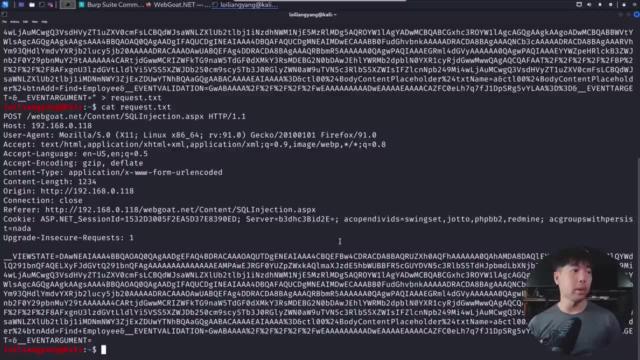 So we have now saved that request into a file. Next up, we can take advantage of this file that we have saved and we can use a tool like, say, SQL Map and we can target this file by entering requesttxt. 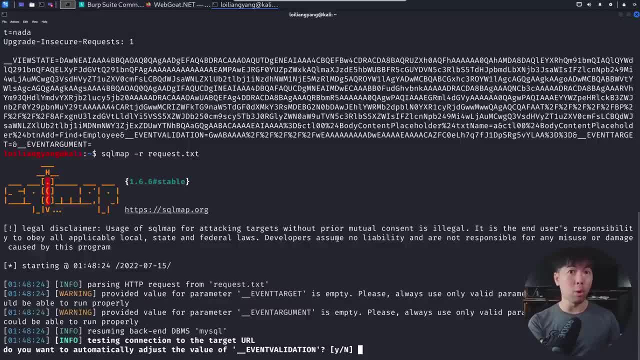 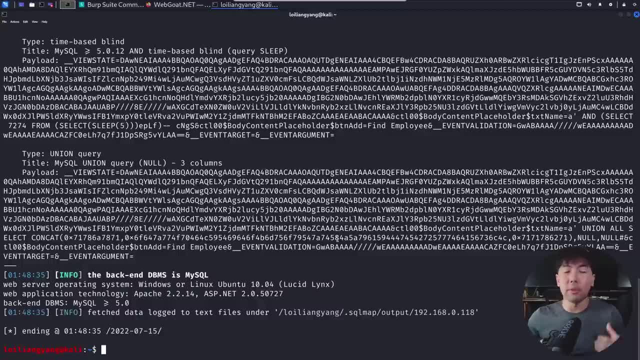 Hit enter on that. and right here SQL Map is sending payloads over into target site so that we can find out where are the different vulnerable parameters that we can go after. And right here we have already ran through the attack and we have logged the file over. 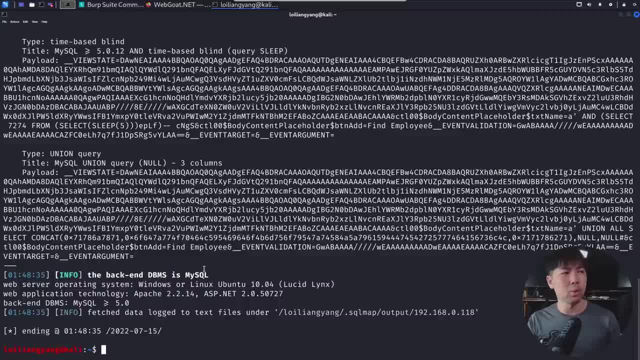 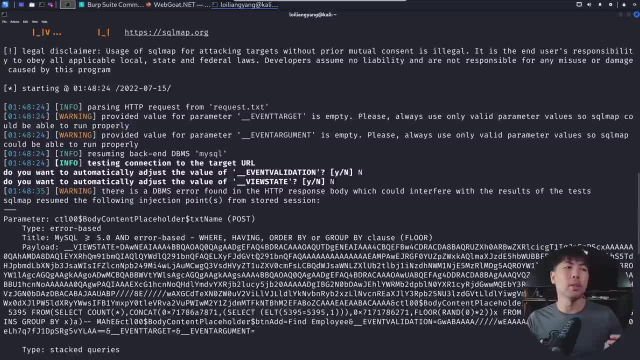 So we can see the following: that the backend database is MySQL And right here we have different MySQL union query. All right, We have time. Big It's blind. And as I scroll up a little further, we can see the different parts of the vulnerable injection points that we can go after. 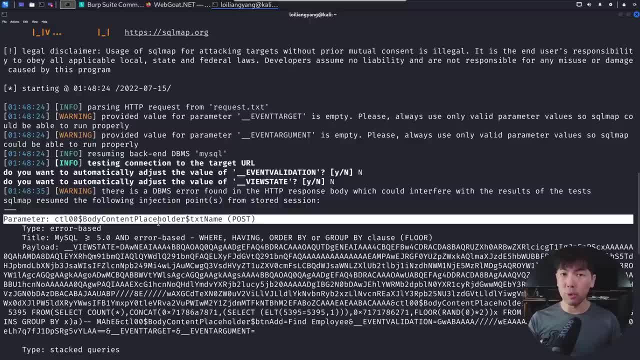 So you can see, here we have the parameters. so body content, placeholder, text, name And, next up, what we can do here is enter SQL Map, and what we want to see now are all the different types of databases within it. 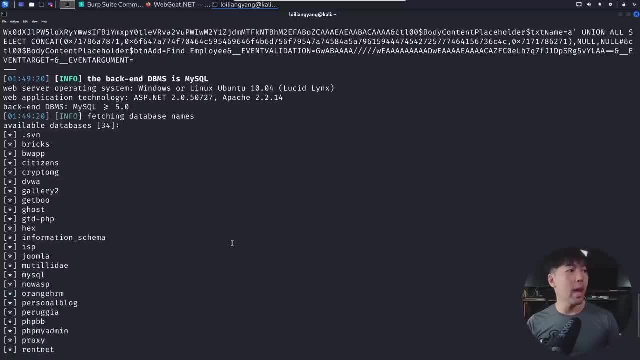 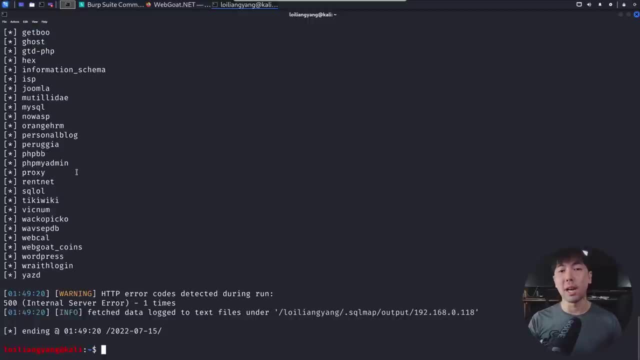 So I can go ahead and enter the following information and we can see right here we have a lot of different databases. So we have Bricks, BWA, BB, All right, We have GetBoo Gallery and all these different databases within it. 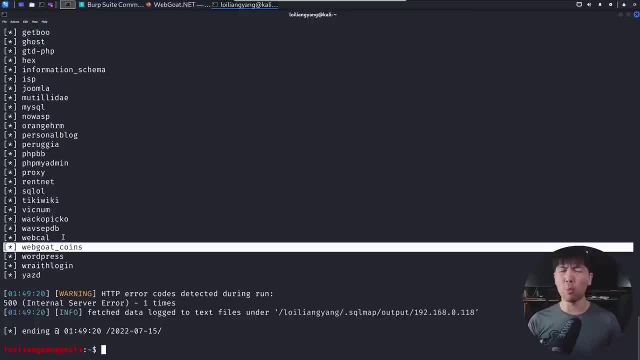 And in this case we have a lot of different databases And in this case we'll be targeting WebGoat Coins and we want to find out all the tables we have in it and to dump out all of that passwords in the customer table. 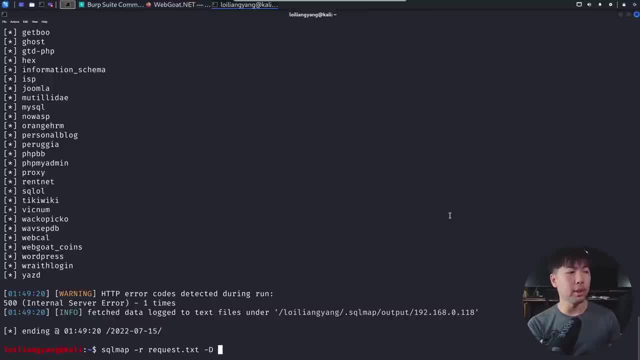 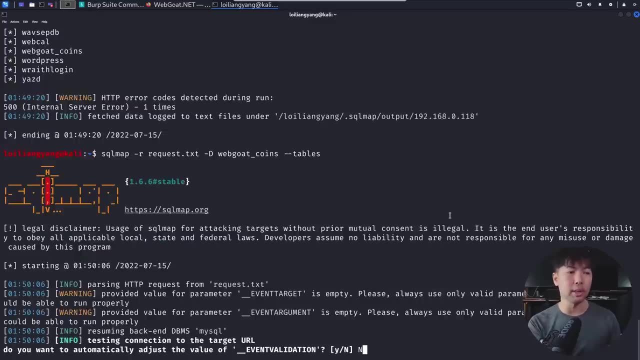 Okay, And all I got to do right now is go ahead and enter the following: All right, So dash D, followed by WebGoat underscore coins, dash dash tables. All right, So this will list out all the tables within this target database. 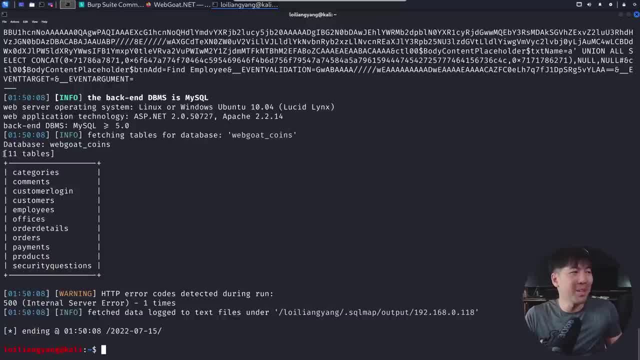 Let's go ahead and do just that, And right here we got a result. This is crazy. Look at that. 11 tables right here, And the one that looks like what we are going after is going to be under customer login. 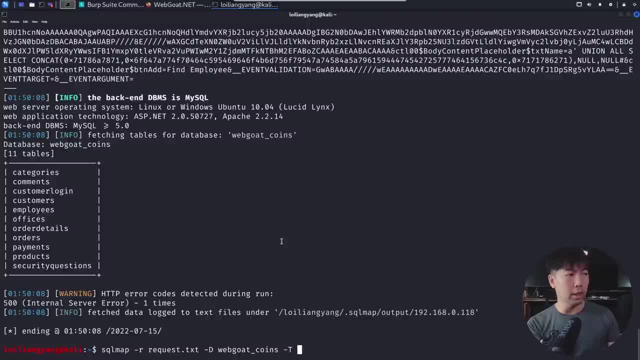 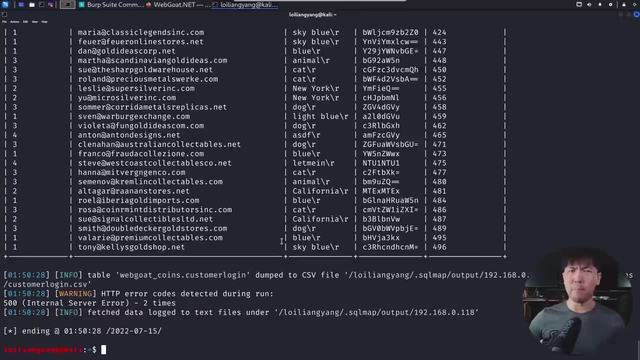 So let's go ahead and do that. So let's go ahead and go after that. So now I can change this over into dash T, followed by customer login, followed by double dash dump. Hit enter on that, All right, And this will give us the opportunity to dump out all of the passwords. 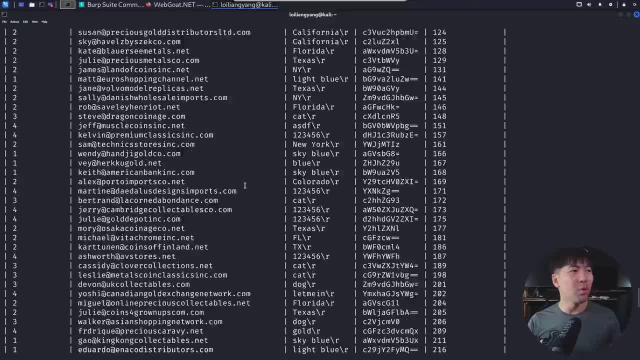 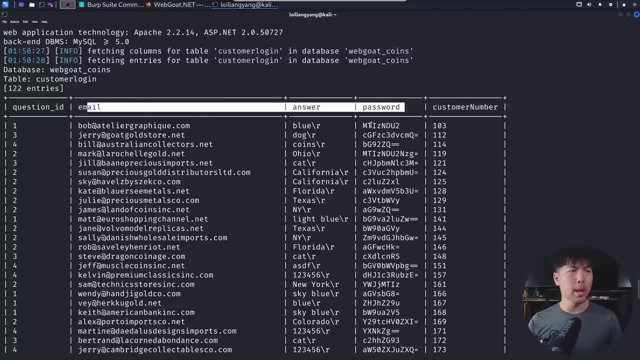 And right here we got it. Look at that. All this of the different email addresses as well as the password field, So you can see here email answer password And right here these are all the different passwords that we managed to find. 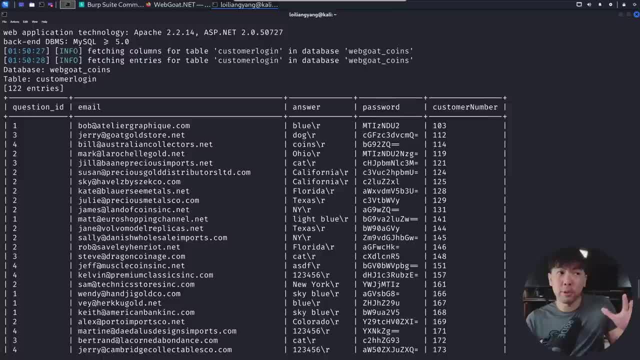 However, it looks a little strange. One thing for sure: These password fields are not hashes, because hashes typically have fixed length, So in this case we can see that there are varied lengths based on the different passwords. This looks like some form of encoding and they look pretty familiar. 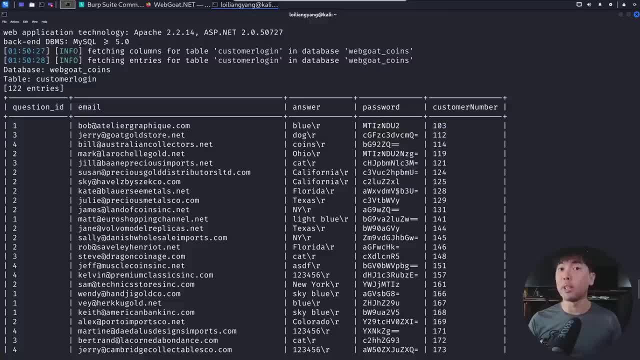 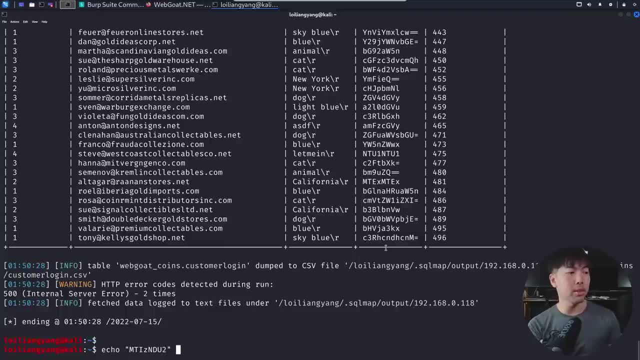 I'm going to go ahead and grab the first password and let's see whether we are able to decode it. So let's go ahead and enter the following: All right, So now what I'll do is go ahead and enter echo, followed by the password that we just copied and paste. 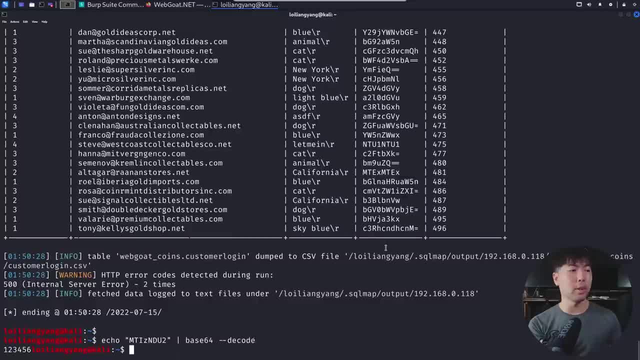 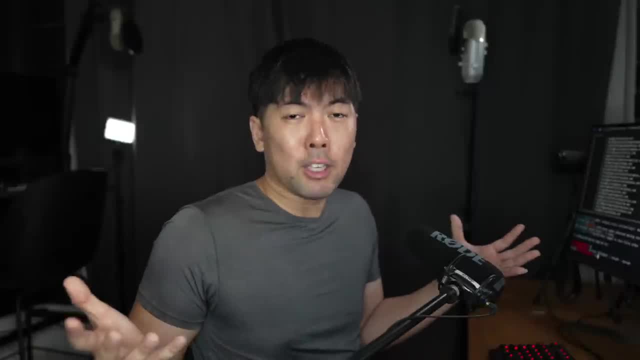 And right here what we can do is use base 64, followed by dash, dash decode, Hit enter on that. Oh, my, look at that. One, two, three, four, five, six. No wonder it looks so familiar, because that is my password. 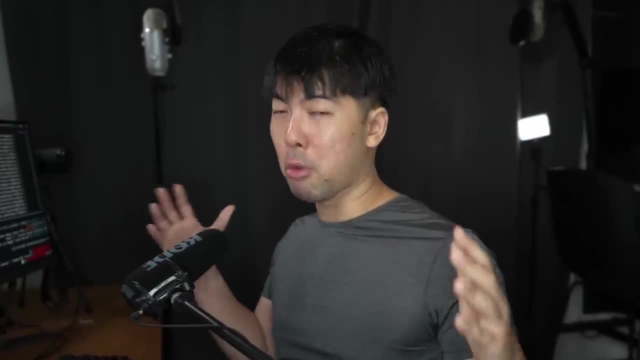 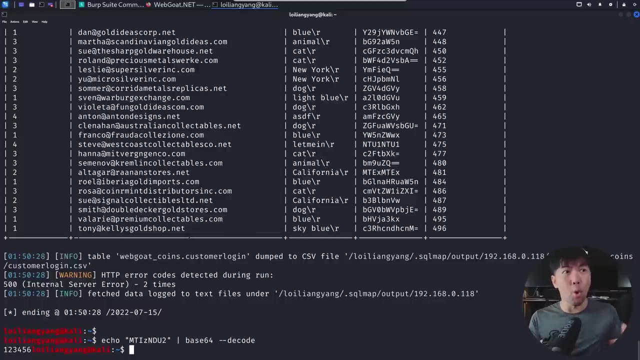 It's the best password in the world. People think that hacker will be using a really complex and strong password, but I choose to do reverse: psychology 101.. And obviously I don't just want one password, I want all of the passes decoded. 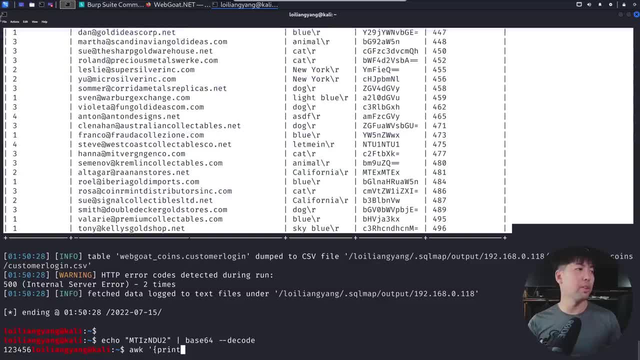 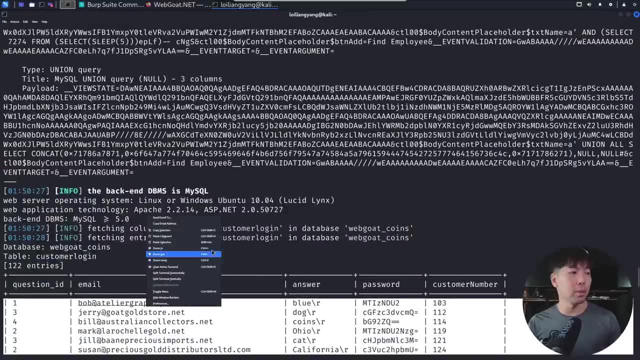 So let's go ahead and do just that. So what I'm going to do now is to save all this different fields into a text file, And after which we can process it, we can change up the format of it and begin decoding them at scale. 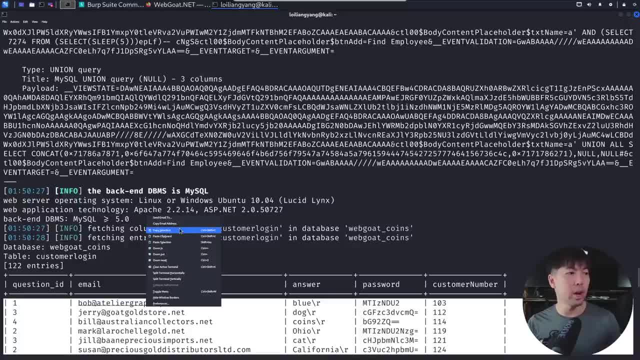 So let's go ahead and copy The whole chunk of it, All right. so let's go ahead and click copy selection. So what I can do now is go ahead and enter echo, All right, followed by all of the information that we have copied. 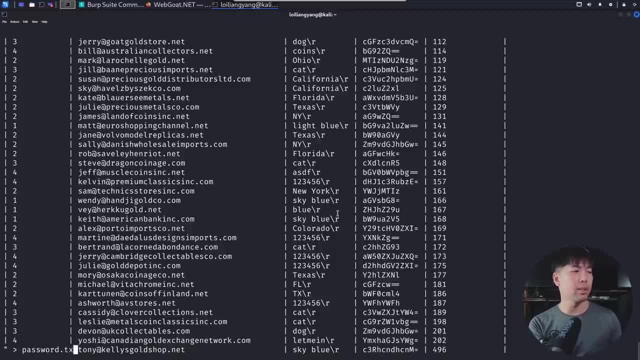 And what I can do next is go ahead and paste them all over into, say passwordtxt, Hit enter on that. All right, I'm going to go clear And I will do a cat passwordtxt And let's see what we get. 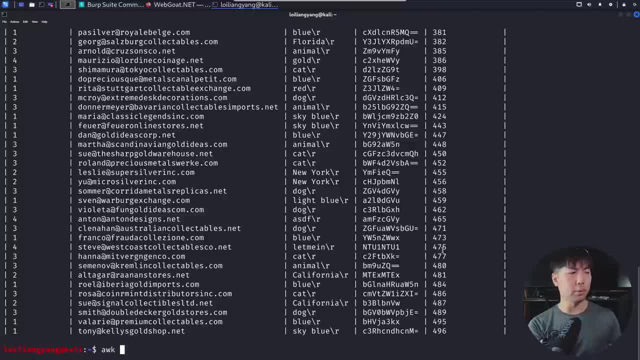 All right. so we got all this different information right here, And what we can do next: go ahead and enter in a bouquet followed by single code, And this case we are going to print number eight- All right, so dollar eight- and then followed by the curly braces. 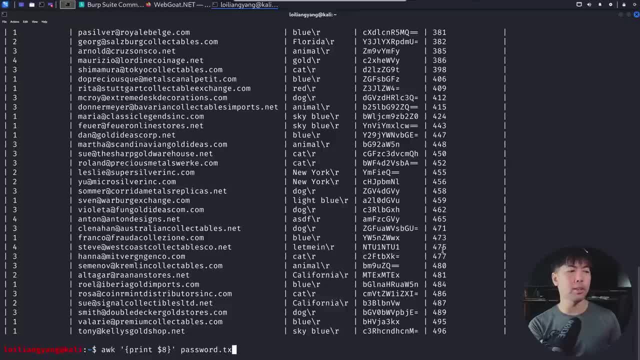 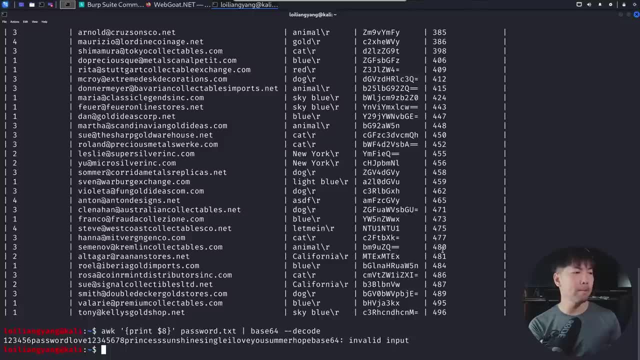 And then what we can do next: go ahead and enter the file. So in this case we have passwordtxt followed by base 64. And then what we can do now is go ahead and enter, say, base 64, double dash decode, hit enter on that. 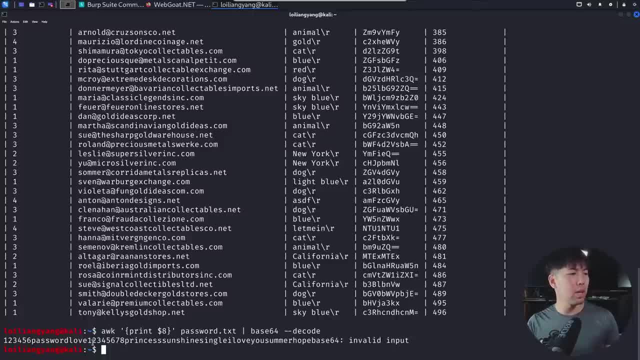 And we got the information All right. so we have one, two, three, four, five, six, password love one, two, three, four, five, six, seven, eight. princess sunshine, I love you, and so on and so forth. 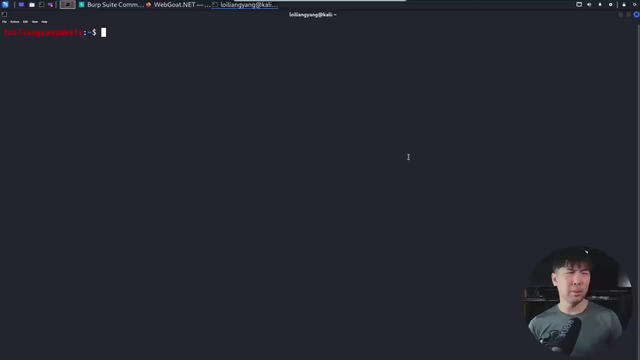 So all of this is different password. However, we do have an invalid input And the reason for the error could be because of a vertical bar. So let's say I go ahead and enter the following, All right, and we can see here. 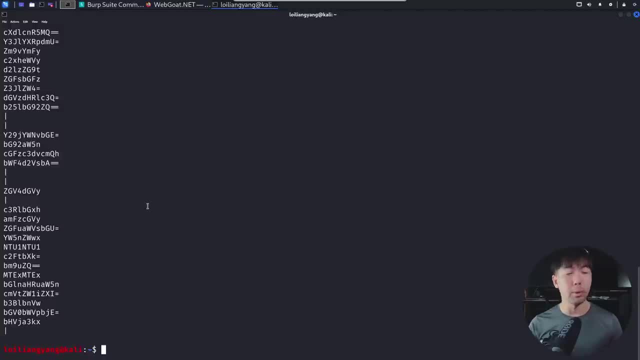 we may have multiple of this vertical bar that may be producing the error. Okay, so for example, if I do the following or I echo with vertical bar and base 64, decode- hit enter on that, we get an invalid input. 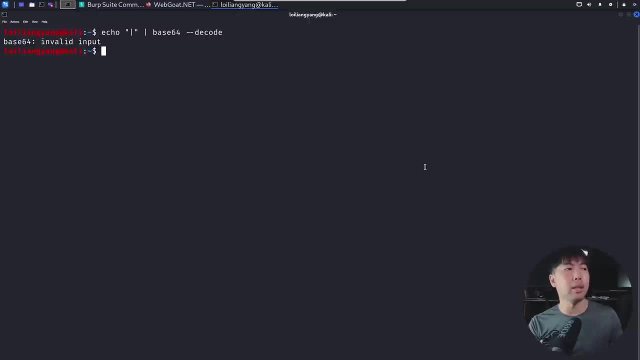 So in that case, what we would need to do is to be able to remove that from the list so that we're able to decode the rest of all those passwords. So let's go ahead and enter the following: All right, so we have the AWK print8, password. 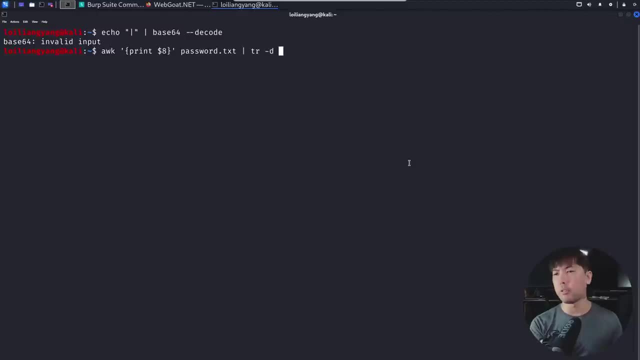 And here, in this case, we want to trim away that. All right. so we have tr-d, followed by the vertical bar again, And now, in this case, we have base 64, dash, dash, decode, And hopefully it works this time around. 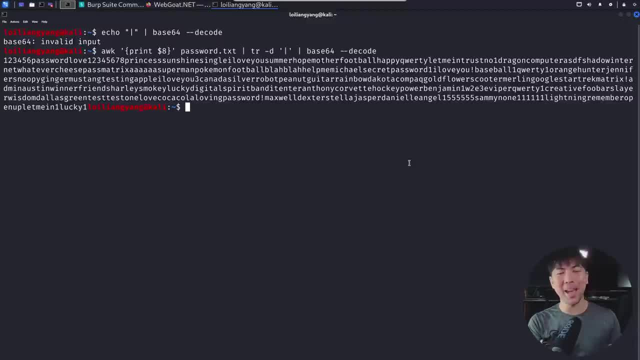 Let's go ahead and hit enter. Hit enter on that, There you go, We got it. We got all of the passwords right here. All right, and of course there's a cleaner way for us to run through the parsing of all those data. 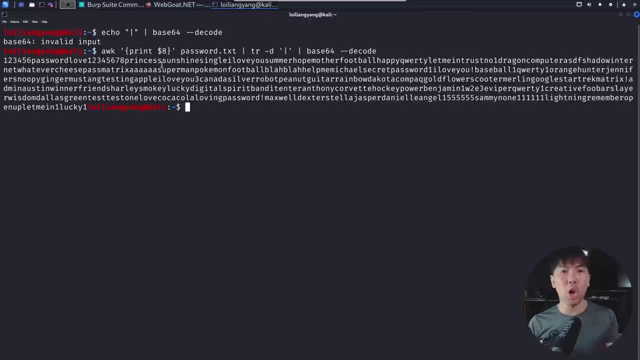 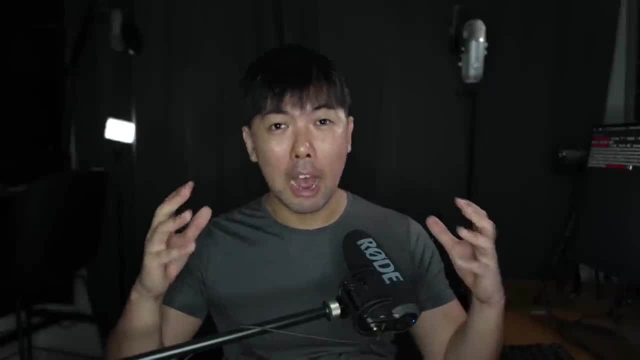 so that we are getting the precision on the password field, the password column, and be able to run through all of that decode. And it's crazily fast, isn't it, How quickly we are able to find vulnerability of a website, after which being able to exploit that vulnerability. 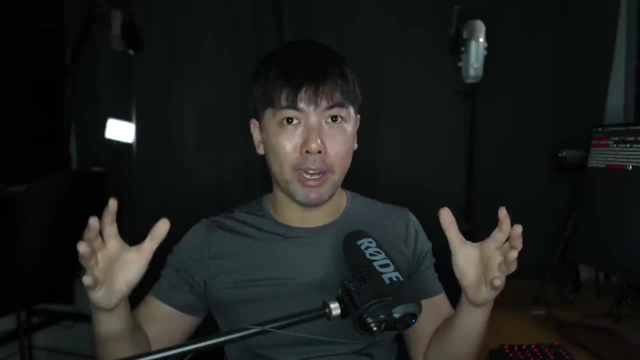 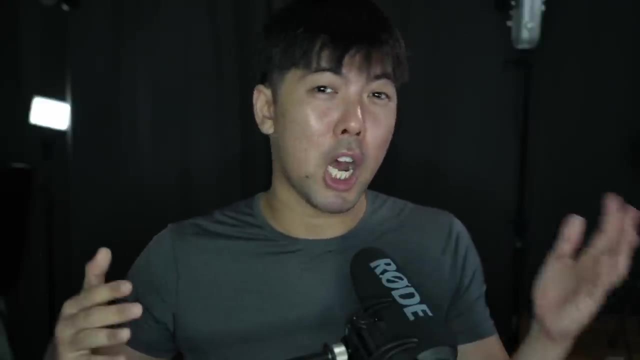 pulling out all of the information from the database system and be able to break all of that passwords. And now that we have the usernames and the password field, we can literally do anything with those accounts. We can try to log into the Gmail, the Hotmail and the Facebook account. 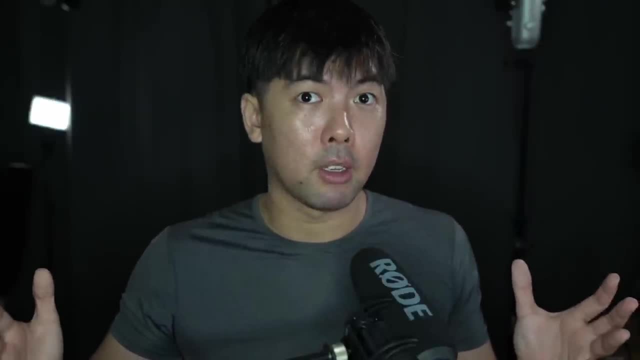 because they could be using the same password across all of these online accounts that they have. Turn on the like, share, subscribe and turn on notifications so that you do not get hacked.